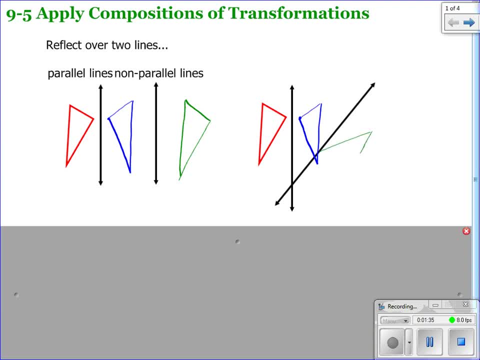 so it's going to look something like this. So what I want down here below is, if you take the red one and look at how it goes to the green one, What did we really do to the object? We slid it to the right, Okay, which is called a translation. 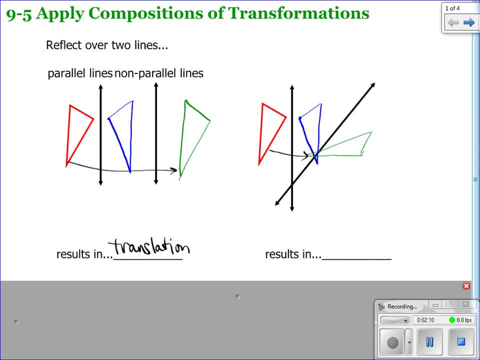 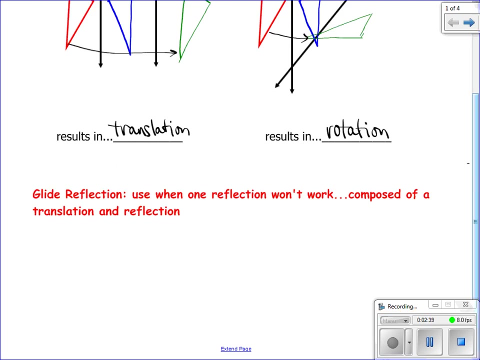 What about if the lines aren't parallel? How did the red one change to the green one? Yeah, it rotated, Okay. Okay. So this isn't anything new. It may look new because you've never seen glide reflection before, But what it's essentially asking you to do is first glide it or translate it slide. 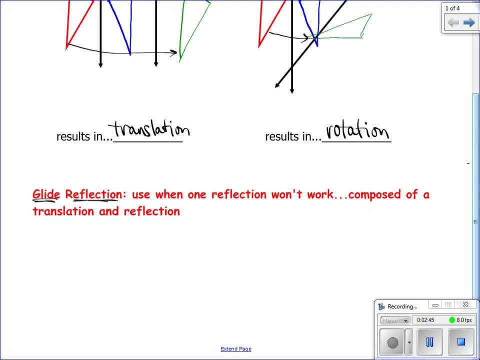 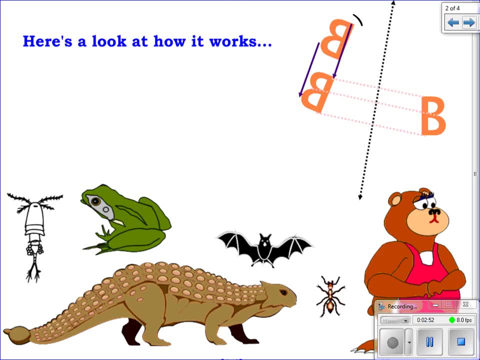 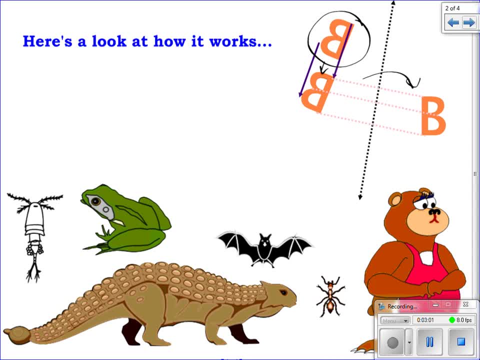 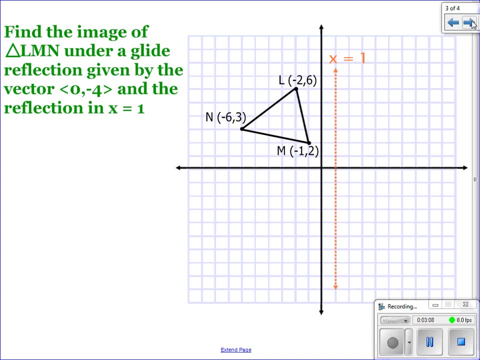 So we're going to practice one of these two step transformations, called composition, on this page right here. Okay, so they're always going to give you the two things to do. you have to do them in the order that they give them to you, or it's not going to end up in the right spot. 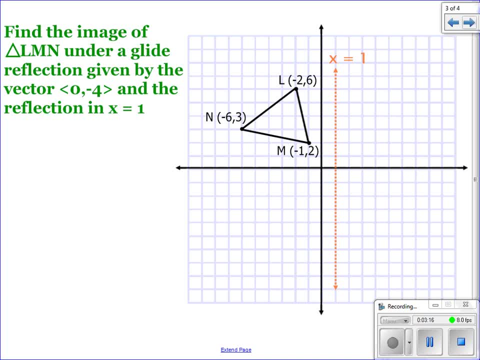 So it says we're going to first slide it and then reflected over this line. Okay, so what direction are we going if we're going along the vector Zero down four, right, the second number is your up down movement. okay, so we're not going left or right. 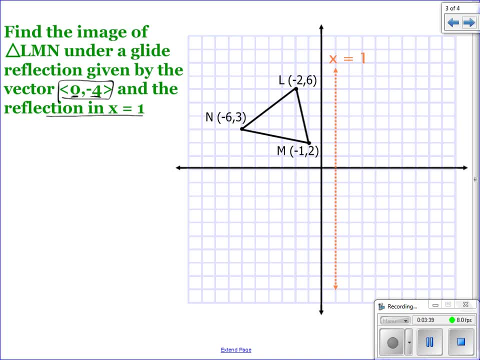 but we are going down four. so the whole triangle needs to move down four units. and we do have to label- if you kids were forgetting the labels with the primes on the quiz yesterday. so that's where our new triangle is and now that we've moved it we need to take 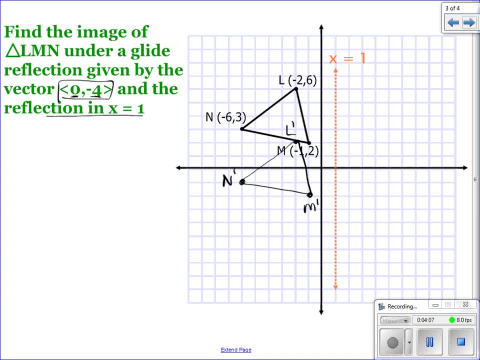 that second triangle, that image, and reflect it over the line they tell us, to which, in this case is x equals, one which i have a little bit of a slip there. so i'm going to point it to the triangle which is going to be the full triangle, and then i'm going to point it to the third triangle. 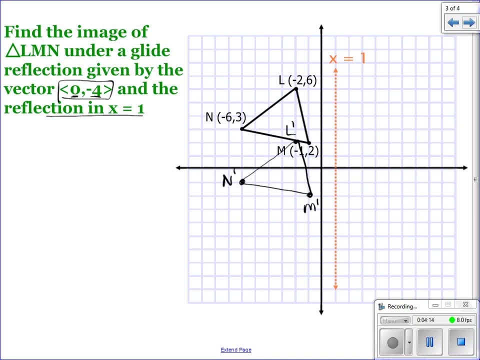 drawn on here already. so a reflection, remember, is just the same distance on each side of the line. so M double prime, because we've done two things to it, is now in this location. L double prime is here and n ends up there. okay, now on the answer key, just to make it very clear on all of your graphs: today I shaded in. 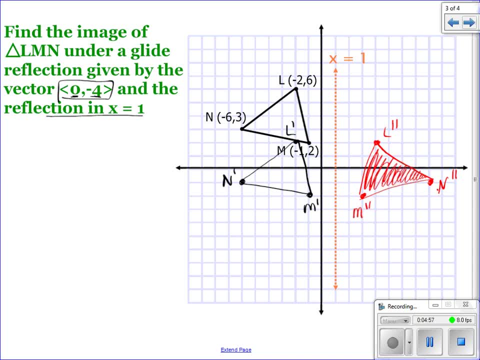 the very final image. so that's where it should end up. make sure you do them in order. it says number one, do this, number two, do this. don't do number two first, okay, otherwise it won't end up in the right spot. questions. okay, so just a. 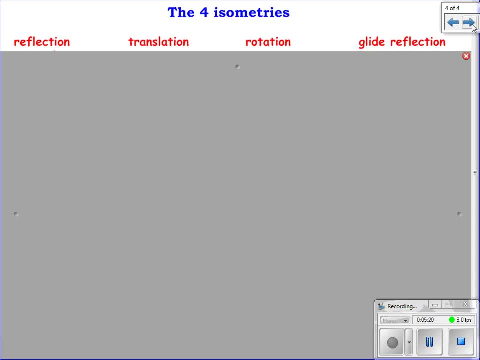 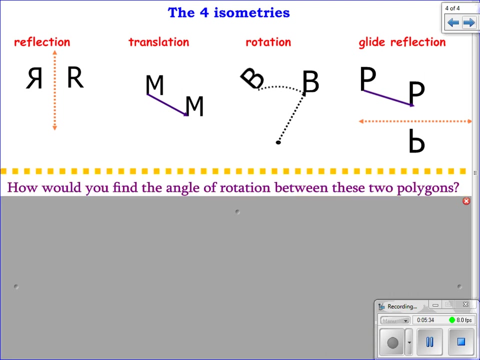 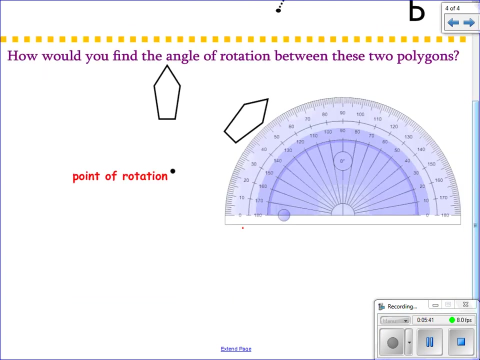 really quick summary of the ones that we have learned so far would be you reflection, translation or slide rotation, and then this new one, which isn't really new, it's just to put together a glide reflection on the test. I might ask you to tell me how much something rotated, okay, which would 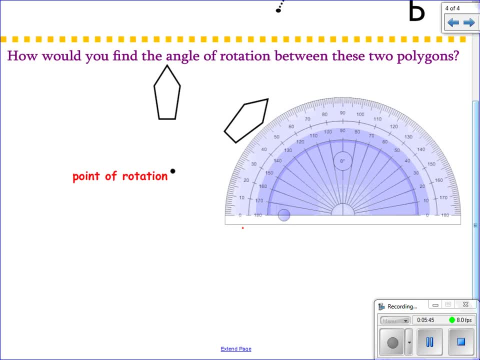 require a protractor. but all you're gonna do- and I'll slide this over on top of here so that you can see it, and I'm not gonna have you all- grab a protractor, but what you're gonna do is you're gonna- this is your protractor, and you're gonna. 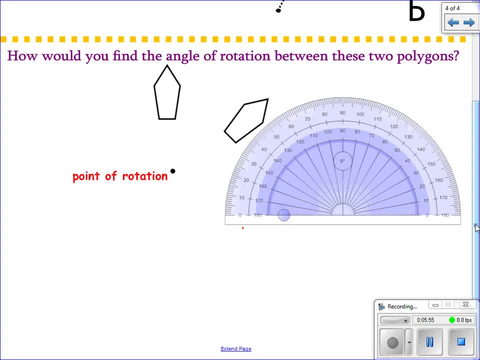 this is your point of rotation, right here. you're gonna connect it with a straight line to any one of the corners on your object. okay, it doesn't matter which one. then you're gonna go back to the point of rotation and connect it to the exact same corner that you picked on the other one. what direction do we?